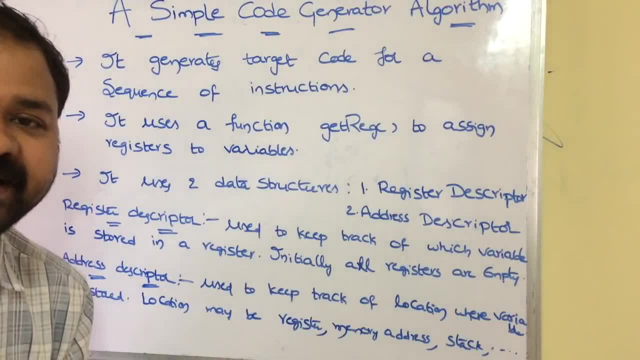 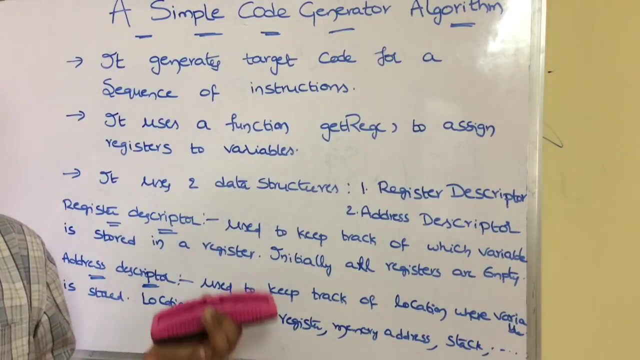 So that means which register contains which variable. The information is provided with the help of register descriptor, So the name itself specifies the meaning. So register descriptor means which register contains which variable And initially all the registers are empty. So that means initially all the registers doesn't contain any variables. 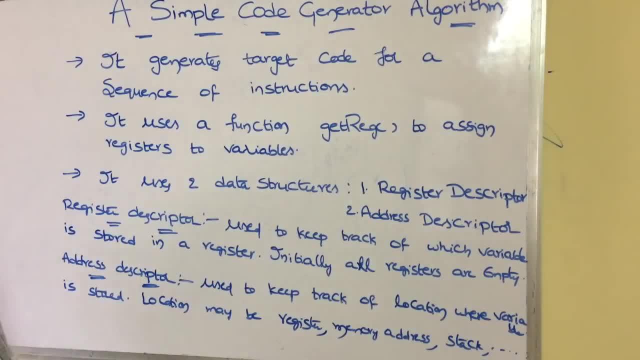 variables and the next one is address descriptor. it is used to keep track of a location where the variable is stored. here the location may be a register, memory address or stack. so address descriptor specifies the variable stores in which location. so the variable may be stored in a register or a memory. 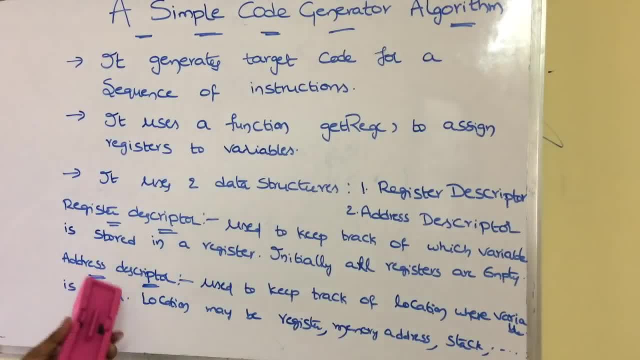 location or a stack. so address descriptor mainly provides variable information. so variable: which variable is stored in a register, or which variable is stored in a memory location, or which variable is stored in a stack. so that is about address descriptor. so what is the difference between register descriptor? 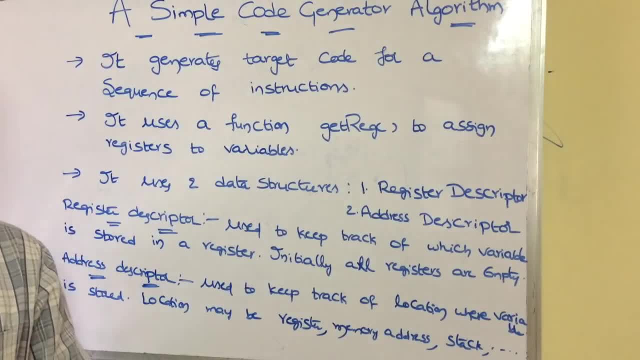 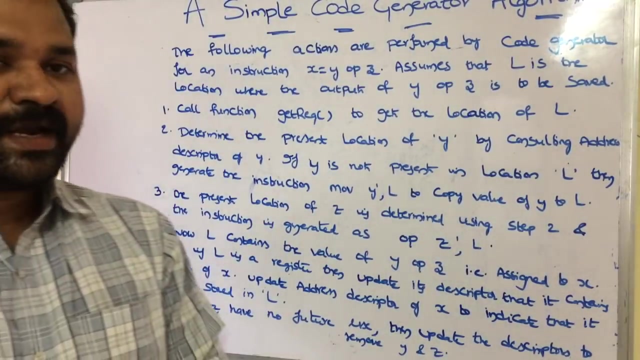 and address descriptor. register descriptor specifies information about register, which register contains which variable, whereas address descriptor specifies location of the variable. that means which variable is stored in a register, or which variable is stored in a memory location, or which variable is stored in a stack. so now let's see a simple code generator. now let's see about a simple. 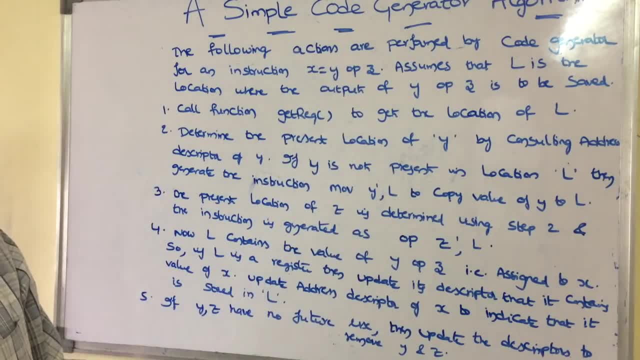 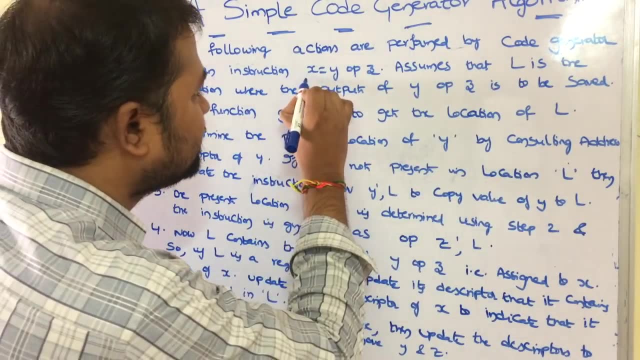 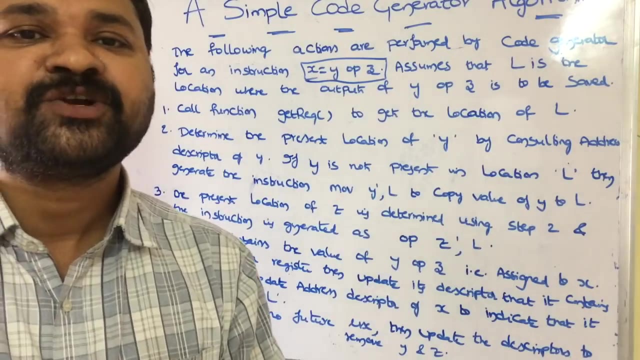 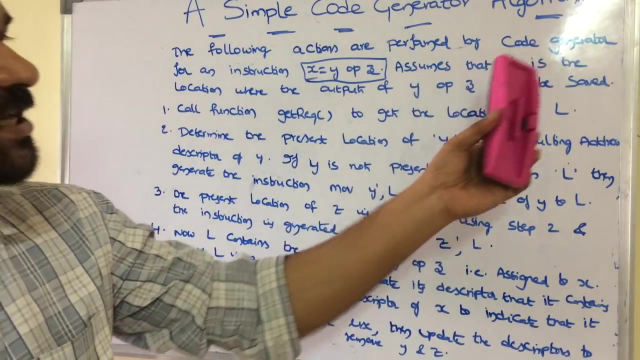 code generator algorithm. let's see the algorithm. here. the following actions are performed by code generator for an instruction: X is equal to Y, OPZ. okay, so here OP specifies the operation to be performed. X, Y, Z are some variables and you can do that by changing the independent function like the function. 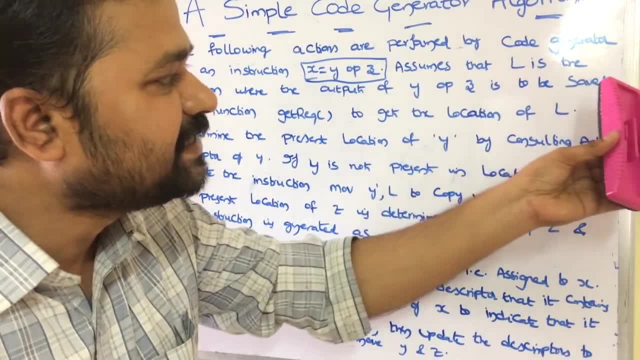 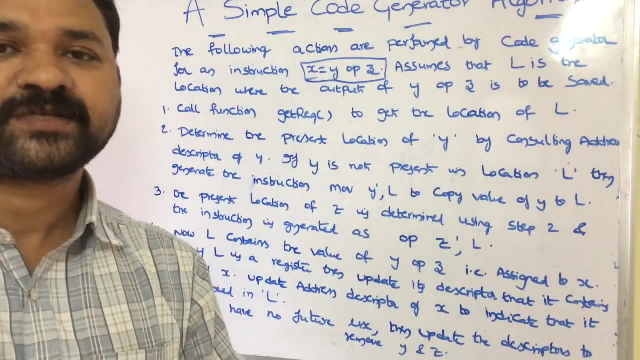 V is equal to V at z的时候, or I get the state of v at such can be perform function to be performed to the external situation using order lock. ok, here, let us assume that here is the location where the output of Y O, P, Z is. 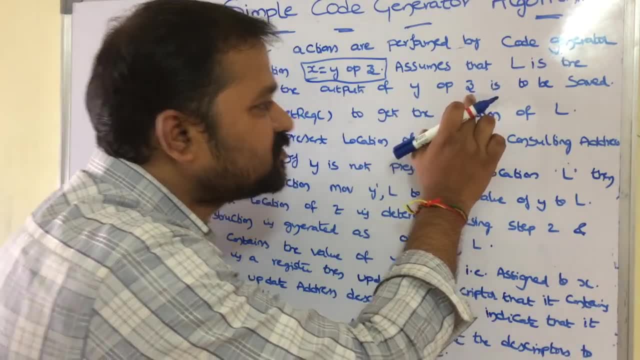 to be saved. so what is OP? it specifies operation to be performed. it may be some addition operation or subtraction operation, like that. so here l is a location where the output of Y OPZ is to be stored. so y contains the result of v. as for this, an action isTo Be 했습니다 In the system 0 if value의â an Orlandopres pigs is l. the output is a location. where is the location? where is the output of yстран ¿of Green R1 is to be Select and White SoenteR Gates in different places in. 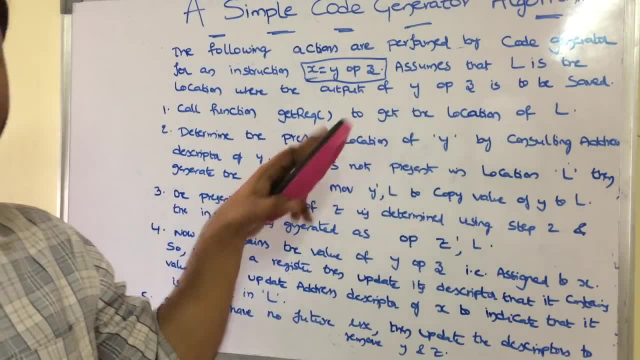 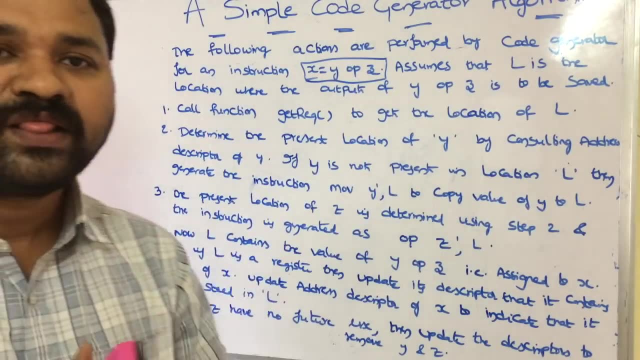 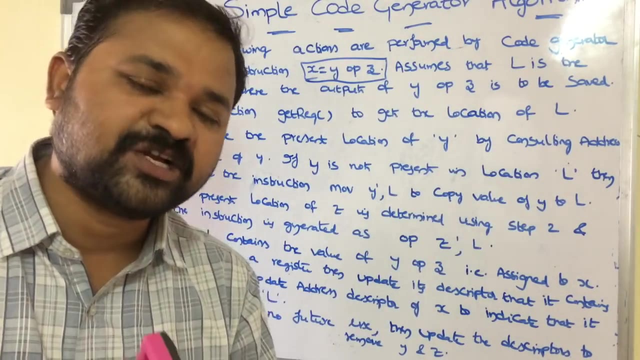 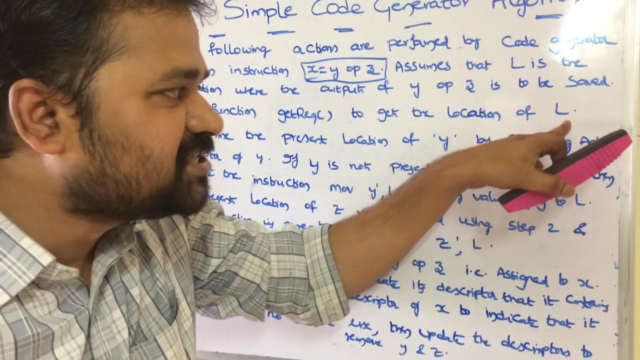 yopz. so let's see the first step here. call the function get. are easy to get the location of l. so call the function get- are easy to get the location of l. so here what is l? l is a location. here the location may be a register or some memory address. so here initially we are using l. 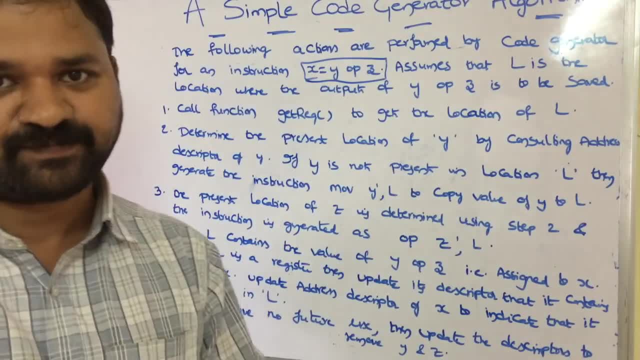 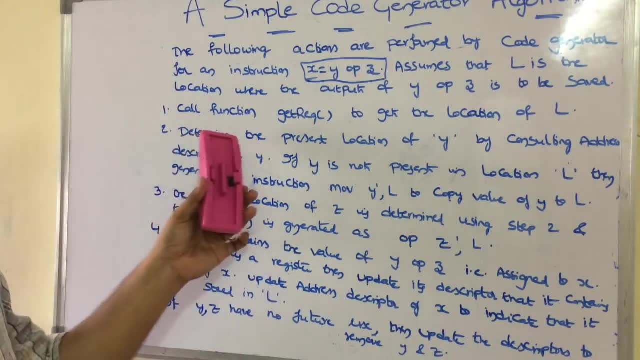 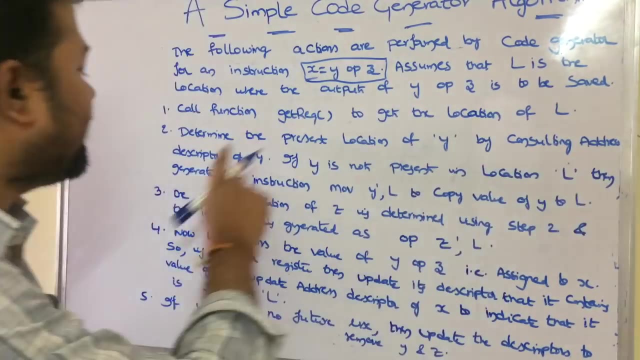 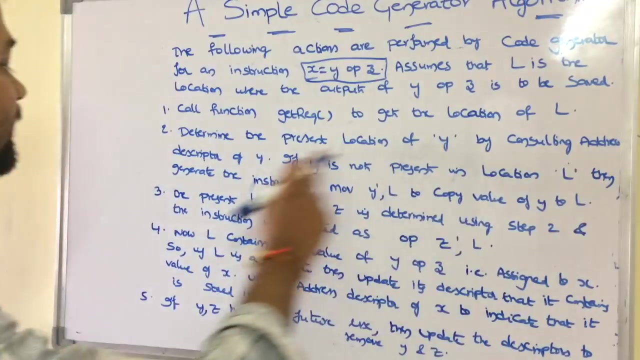 for storing the result of yopz. so, after performing all the operations, l contains the result of yopz. now let's see the second step. determine the present location of y by consulting address descriptor of y. if y is not present in the location l, then generate the instruction: move y. 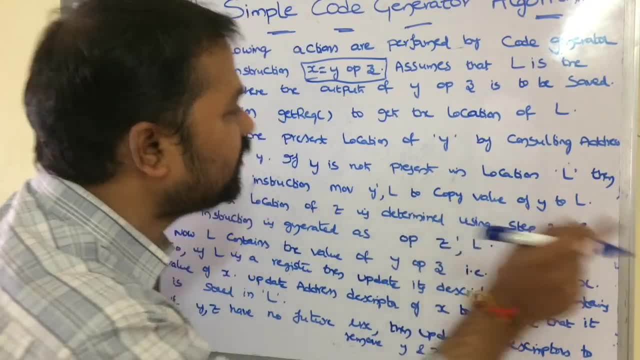 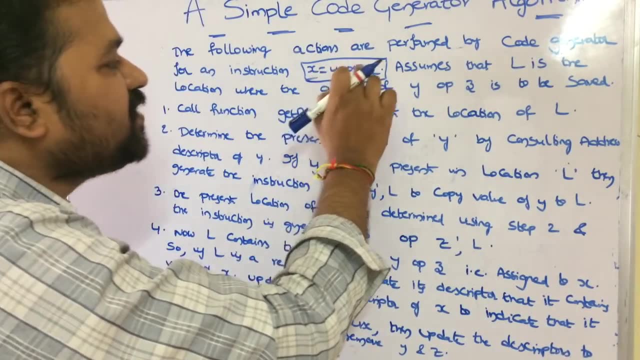 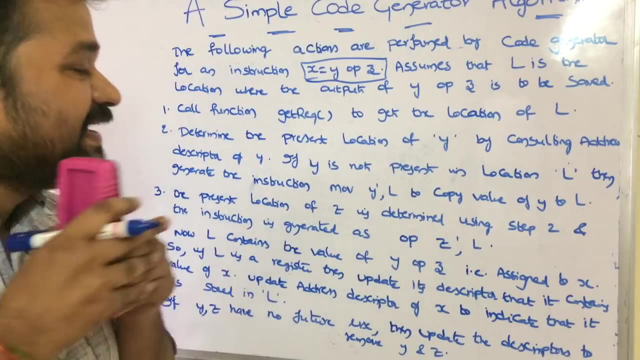 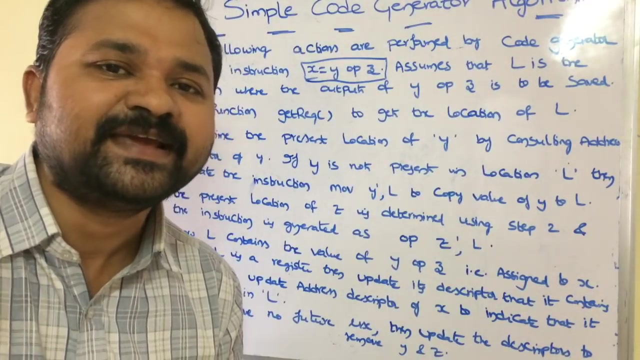 dash comma l to copy the value of y to l. so here, uh, here we have y. here, okay, in the right hand side we have yopz. so first we have to determine the location of y. so for that purpose we need to check whether y is available in any location or not. if y is available in any location, 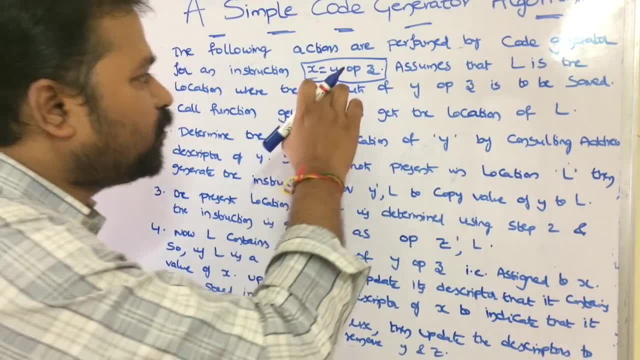 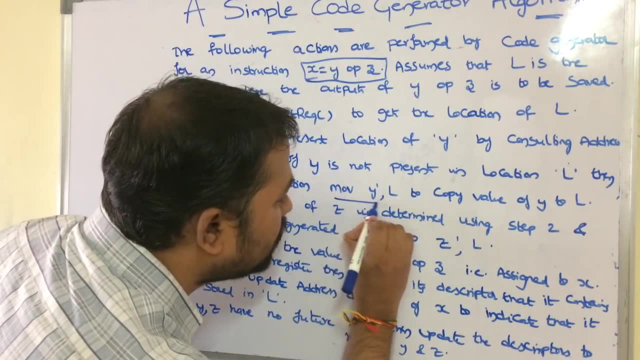 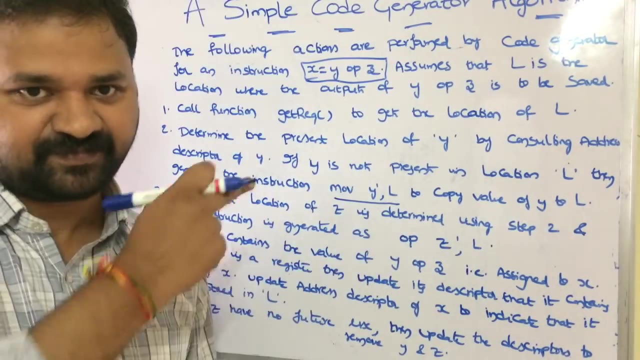 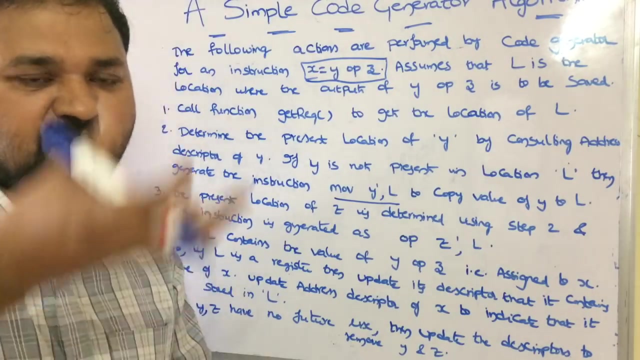 then there is no problem, we can use that location. suppose, if y is not available in any location, then we have to generate an instruction called move y, dash y prime comma l. here y prime means wise address descriptor. so what is address descriptor? it contains the location or the location where the variable is stored, so the corresponding 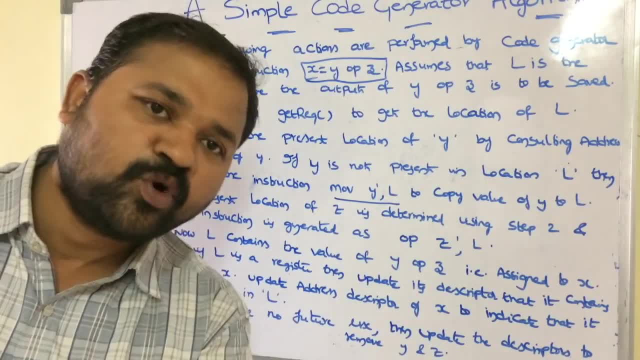 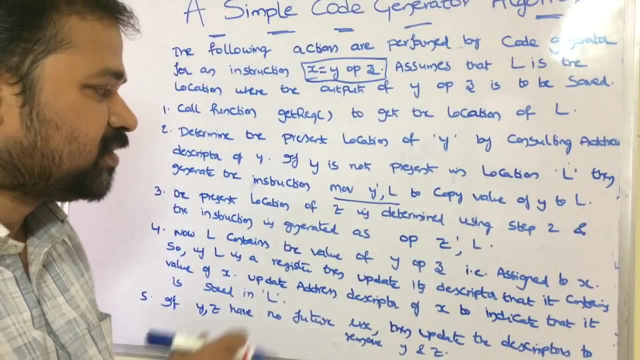 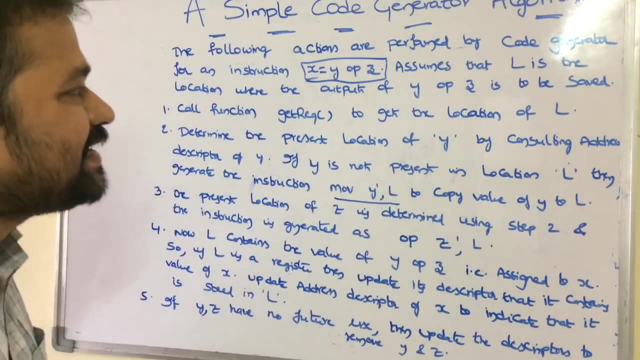 variable may be stored in some register or some memory address or some stack. okay, so this y dash contains that value of y. okay, so move the y dash contains the value of y. so move the value of y to l. so now l contains the value of y. okay, so what is the second step here? 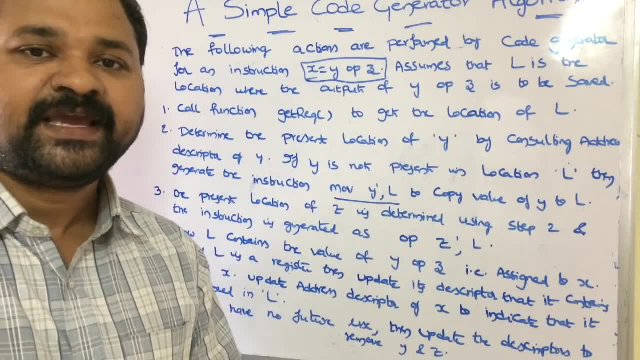 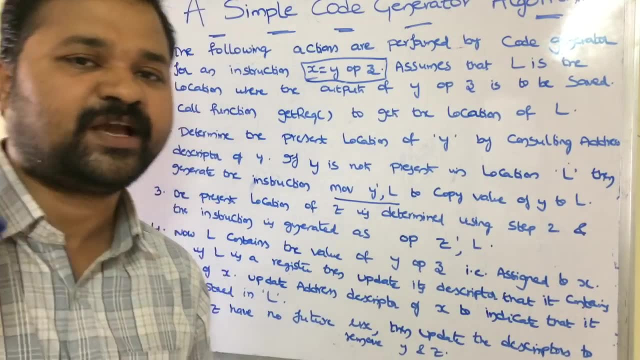 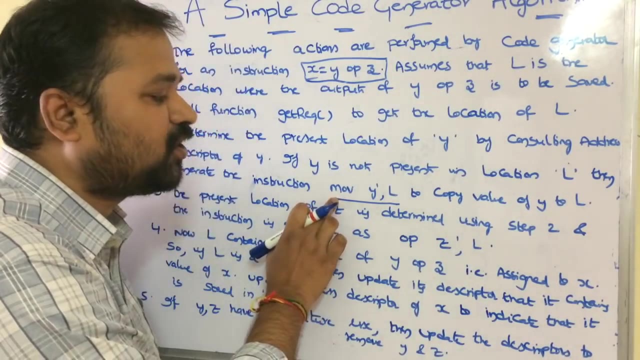 we need to determine the location of y. if y is already available in any one of the location, then there is no problem. directly we can access that location. suppose, if y is not available in any one of the location, then we have to generate an instruction called move y dash comma l here. 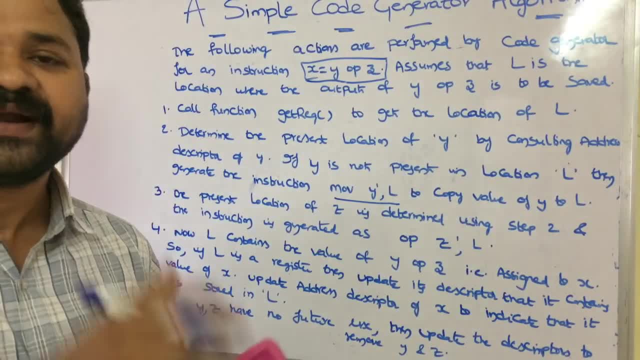 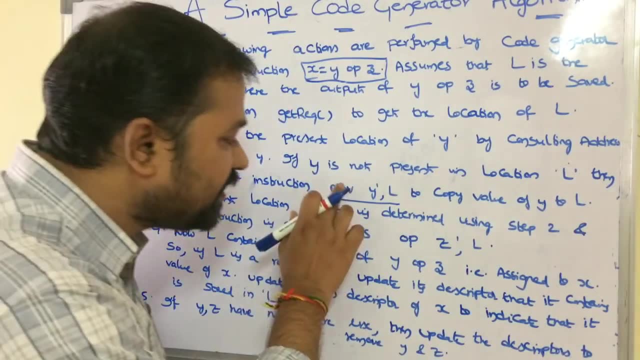 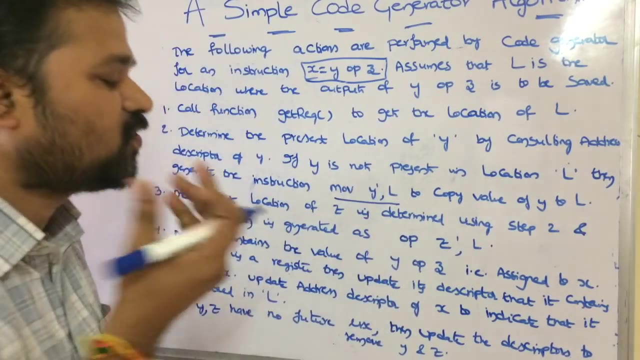 y prime specifies address, descriptor of file. so address descriptor of y contains the location of y, so in which location it is stored. okay, so by executing this instruction we can copy the value of y to here. so y dash contains the copied value of file to a location n. so in the same way, let's see the third instruction. 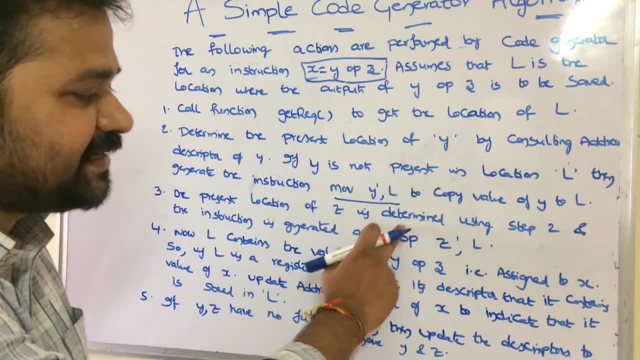 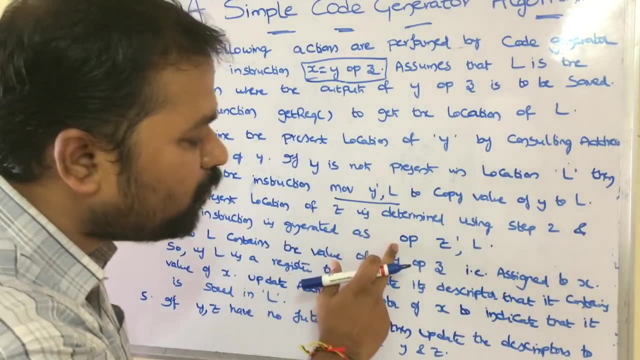 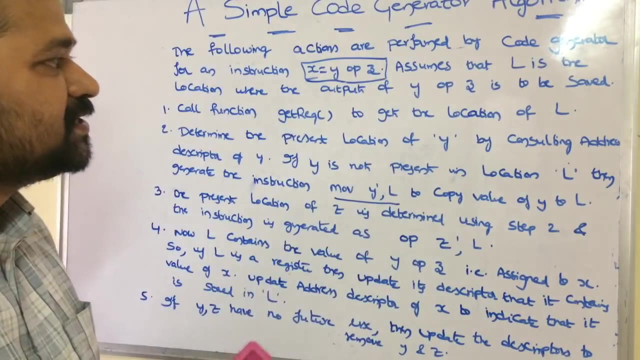 the present location of z is determined using step 2. so this is nothing but step 2, and the instruction is generated as op z dash comma n. so in the same way we have to determine the location of z. so if z is available in any one of the location, then there is no problem. 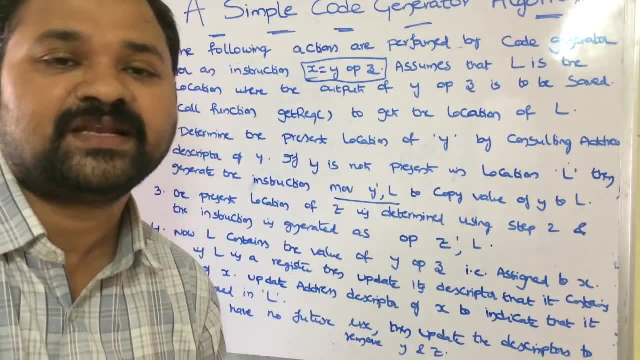 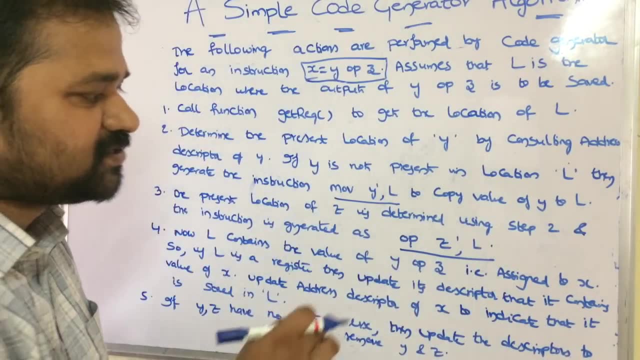 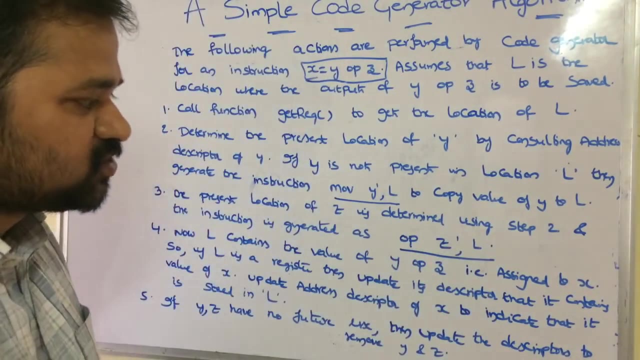 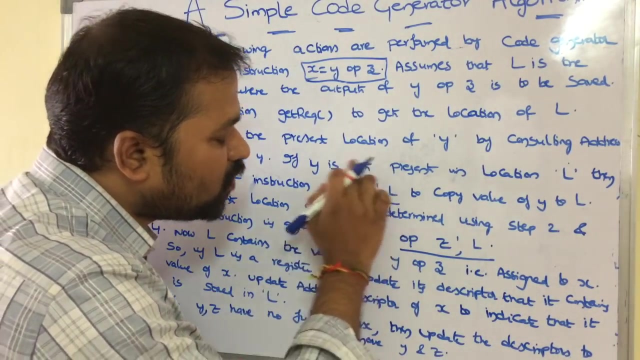 whereas if z is not available in any of the location, then we have to execute an instruction called op z dash comma n. so here, z dash specifies address descriptor of z. so it contains the copied value of z. so the copied value of z is moved to l now. so now one l contains the copied value of y. 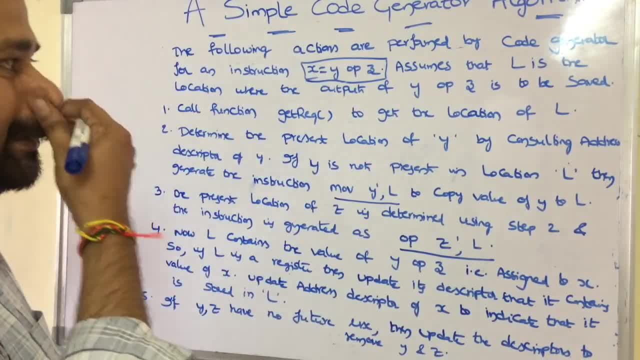 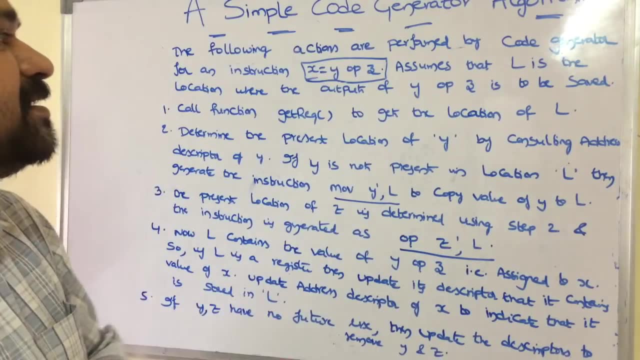 and the second, l, contains the copied value of z. so so, so, So that we can perform operations on one location of y and another location of z, So a result may be generated, and that result is assigned to x. Now let us see the fourth step. 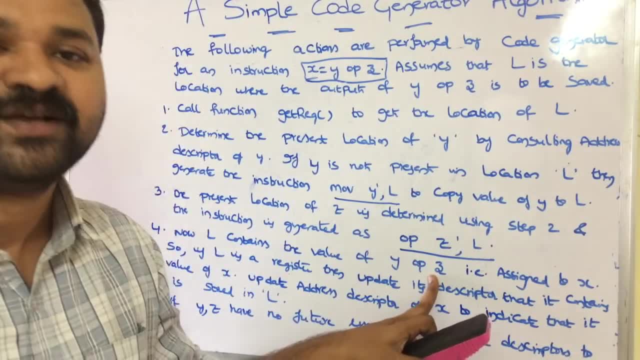 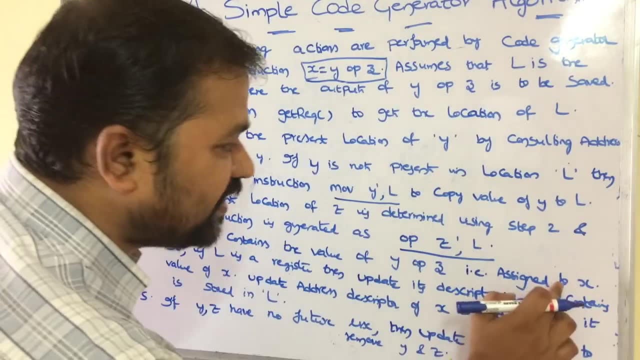 Now, l contains the location of y, o, p, z, So after performing this operation we may get some result. That result is stored in l, So l contains that location. So that is assigned to x. So here, what is the left hand side variable, x? 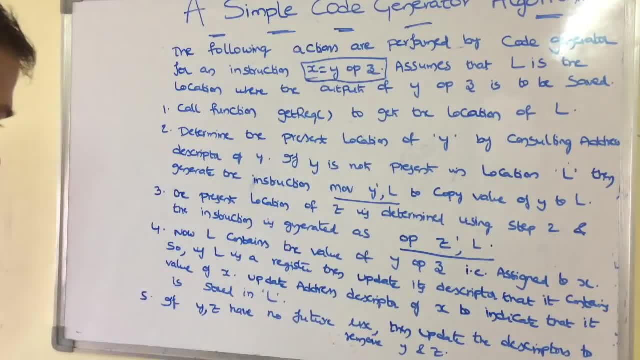 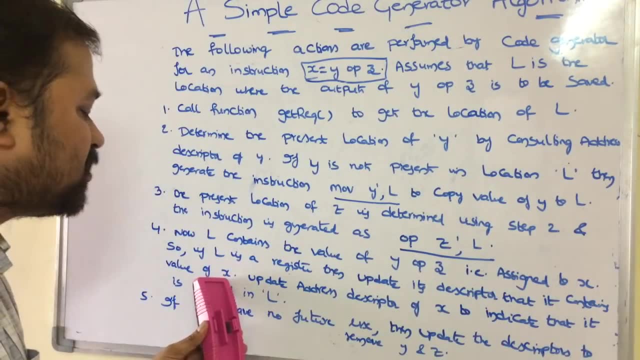 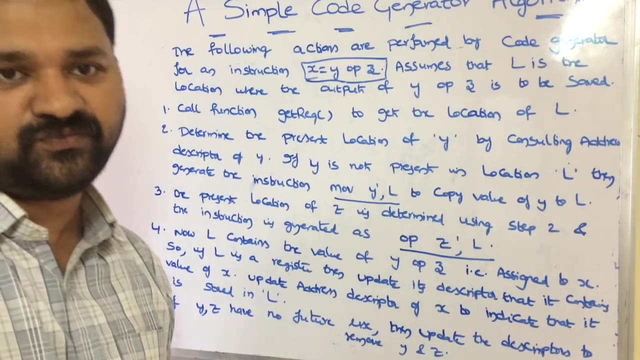 So we have to store the result of y, o, p, z in x. So if l is a register, then update its descriptor that it contains the value of x. So if l is a register, then we have to update its register descriptor so that we know that it contains the value of x. 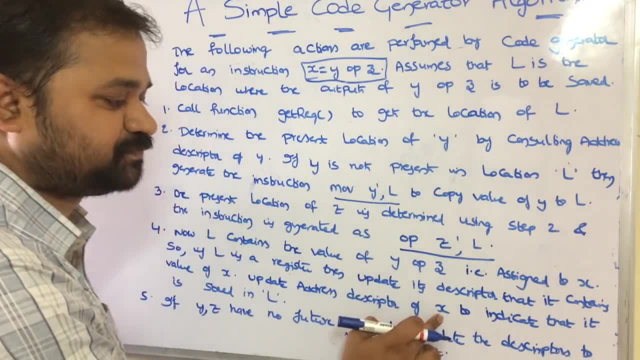 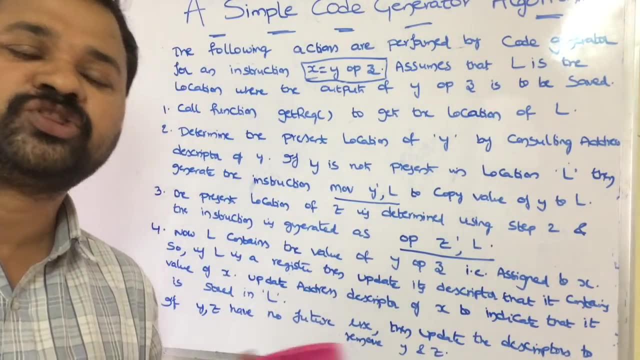 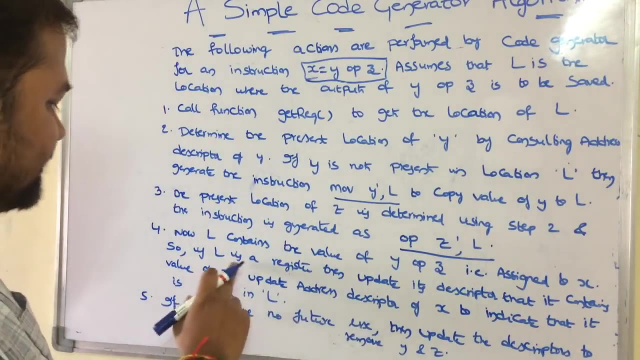 So likewise, update address descriptor of x to indicate that it is stored in the location l. So we need to update both address descriptor as well as. So if l is a register, then update its descriptor that it contains the value of x. 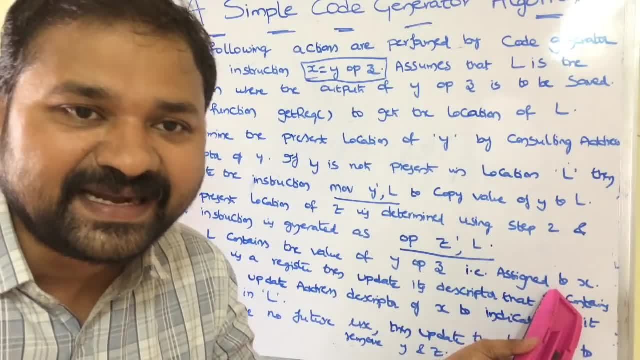 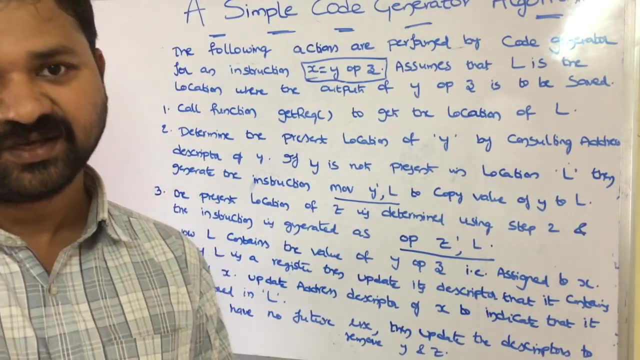 Update address descriptor of x to indicate that it is stored in the location l. And the last point here is: if y, z have no future use, So often, After performing, after executing this instruction, if there is no use of y and z in the future, 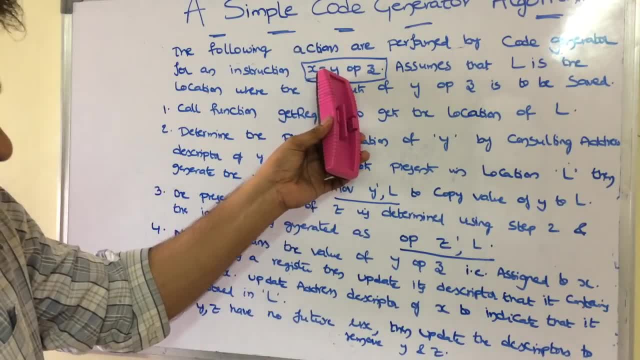 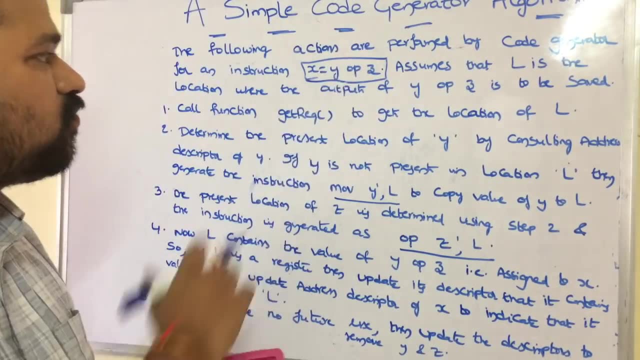 then we can update both the register descriptors y and z, both the descriptors y and z, to remove y and z. Why? Because there is no need of y o p z in the future. So here mainly we have three steps here. 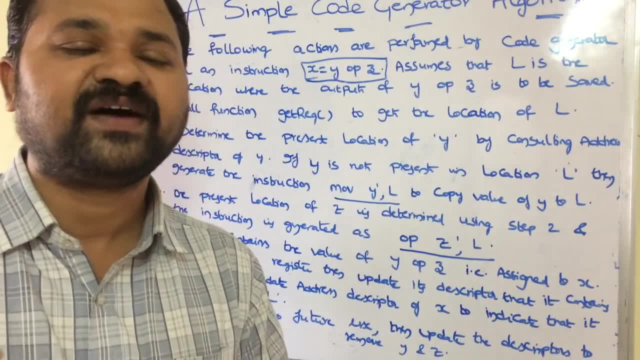 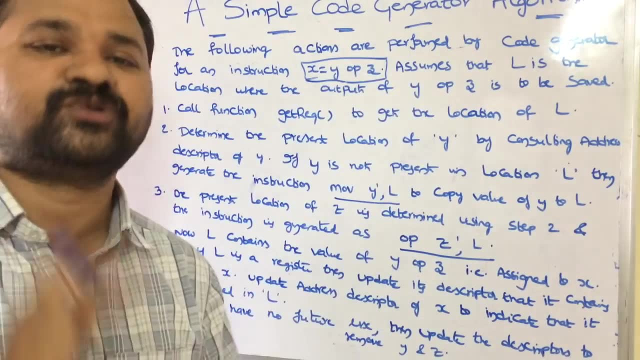 Five steps here. The first step is we have to call a function called getRez in order to get a location where the result of y o p z is to be stored. And the second step is we have to check whether y is available in any one of the location or not. 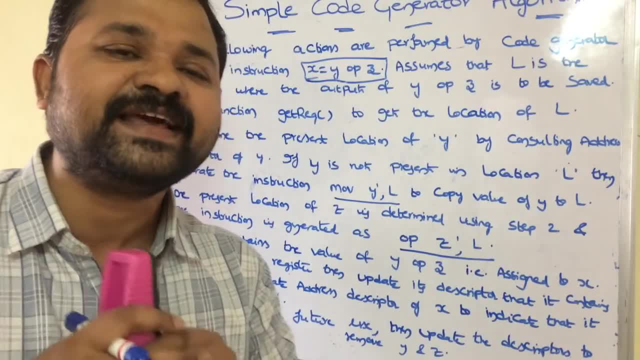 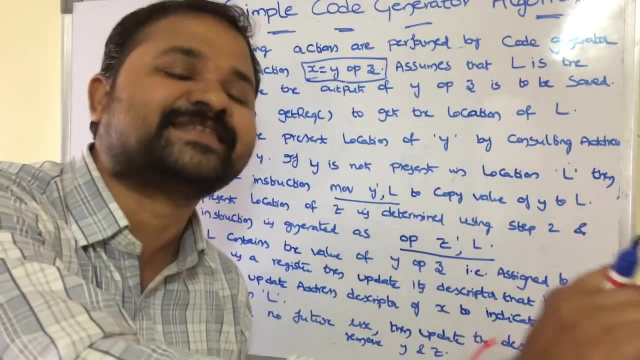 If it is available in any one of the location, then there is no problem. Suppose, if y is not available in any one of the location, then we have to consult its address descriptor, Okay, And execute an instruction called move y dash comma l. 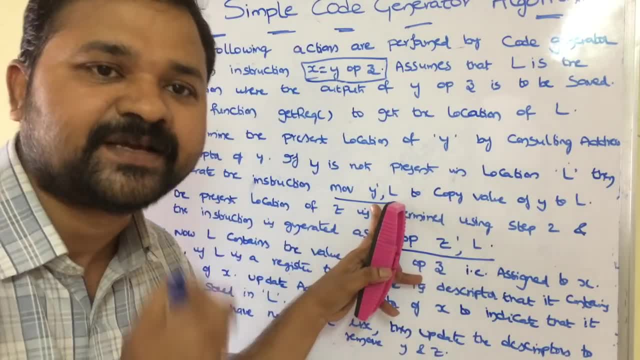 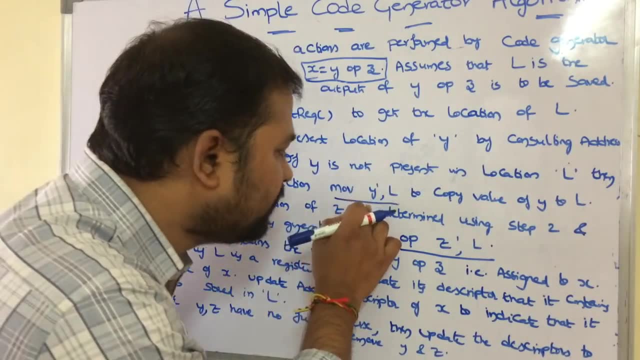 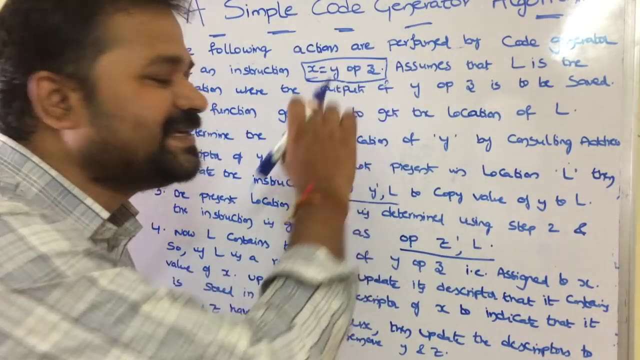 So here y dash is an address descriptor which contains the copied value of y. So by executing this instruction, We can copy, we can assign the value of y to l. In the same way, in the next step we have to check whether z is available in any one of the location or not. 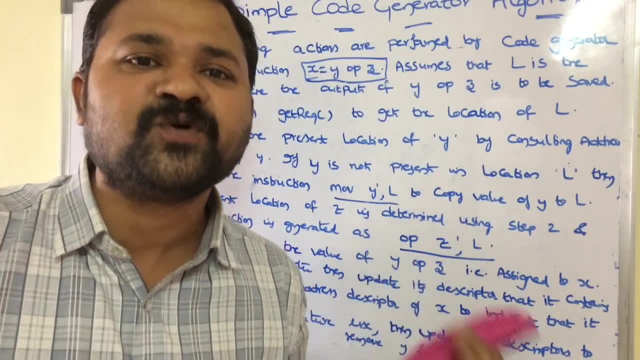 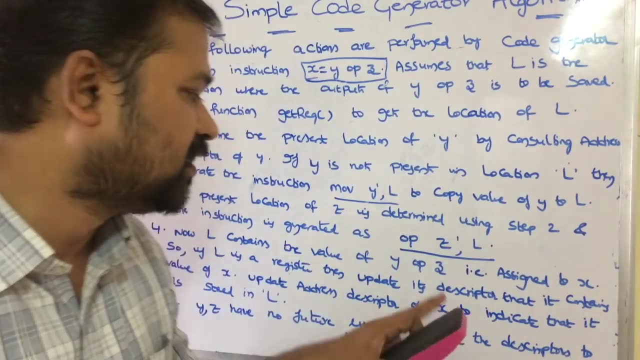 If z is available in any one of the location, then there is no problem. Suppose, if z is not available in any one of the location, then we have to execute an instruction called op z dash, comma l. So z dash specifies address. descriptor of z. 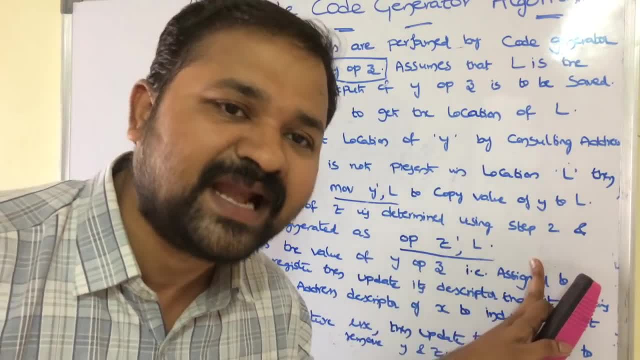 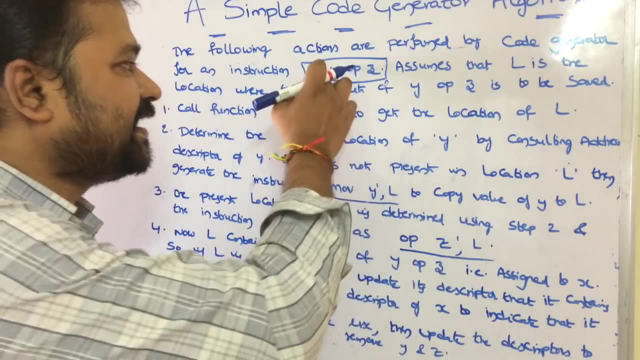 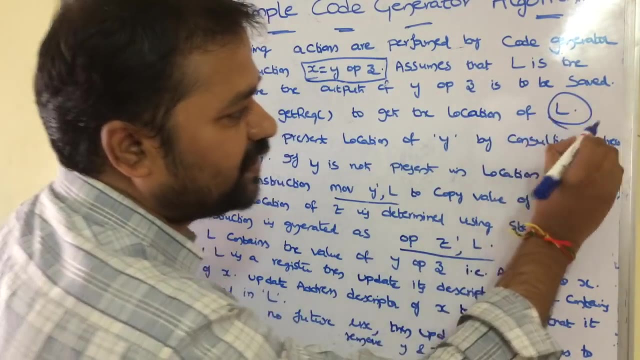 So the copy is done. Okay, So the copied value of z is moved to l now. So now we know the location of y as well as the location of z. So that execute this instruction. So, after executing this instruction, the corresponding result is stored in this location. 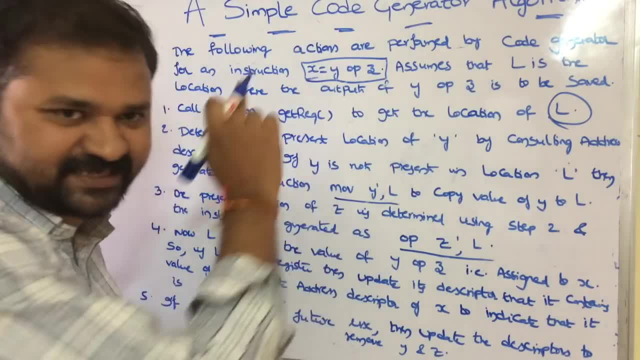 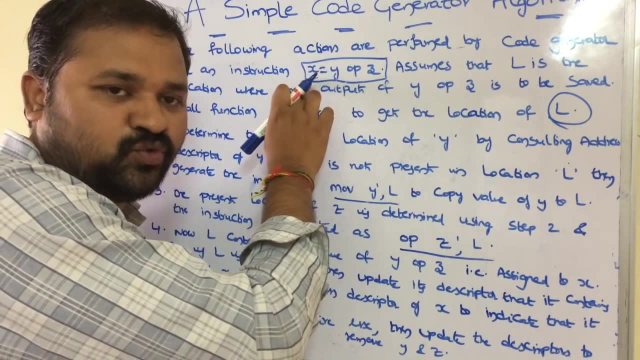 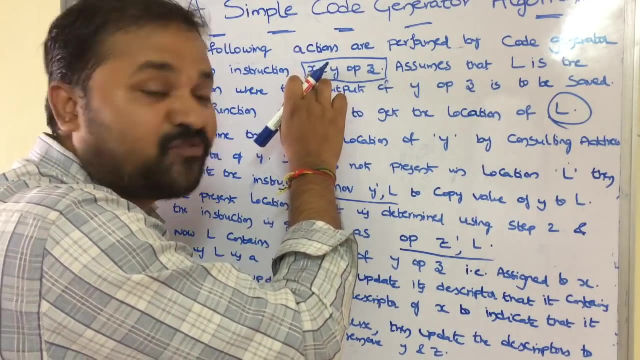 Okay, And that value is to be stored in x. Now we have to update register descriptor as well as address descriptor. So we have to update the register descriptor of l So that it specifies that that register contains the value of x. 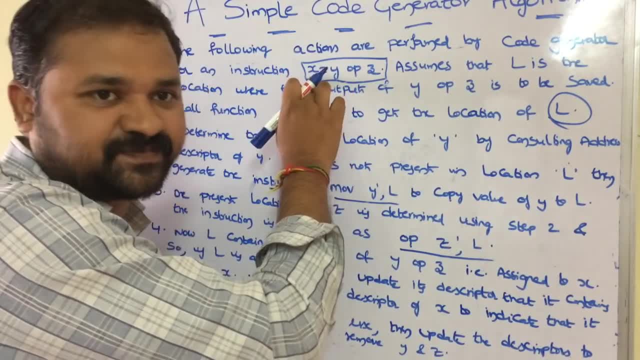 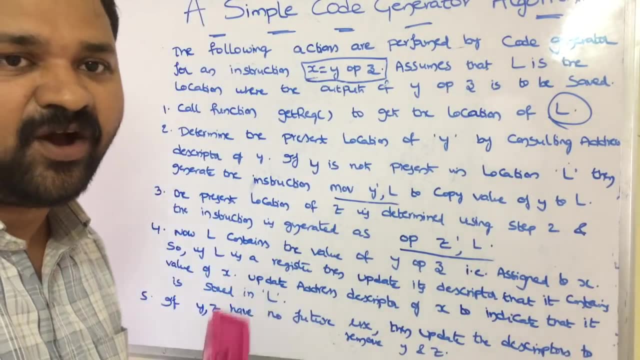 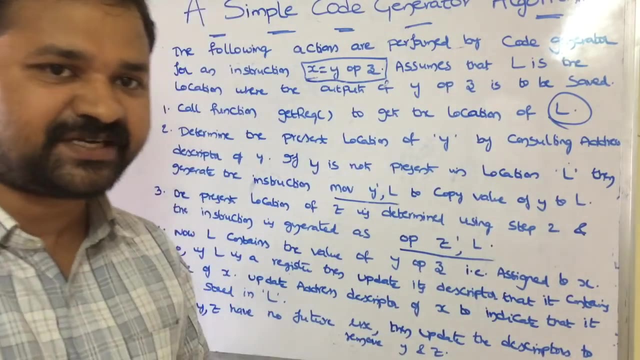 So likewise we need to update address descriptor of x So that it specifies that this x is to be stored in the location l. Then after that, the last step is: if there is no future use of y and z, then we can update those registers by eliminating y and z from the registers. 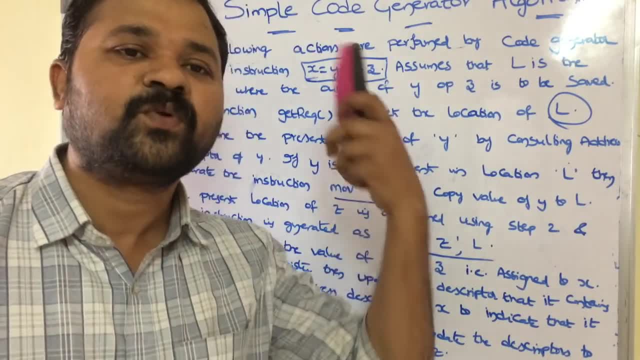 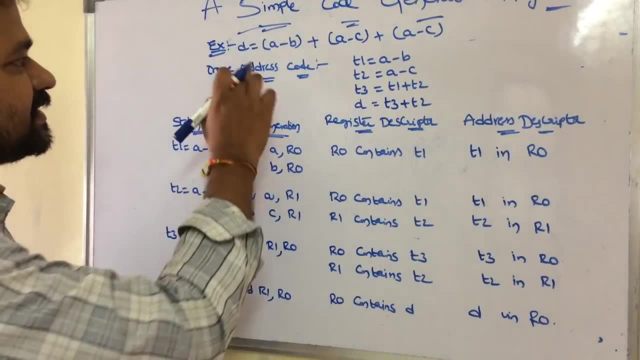 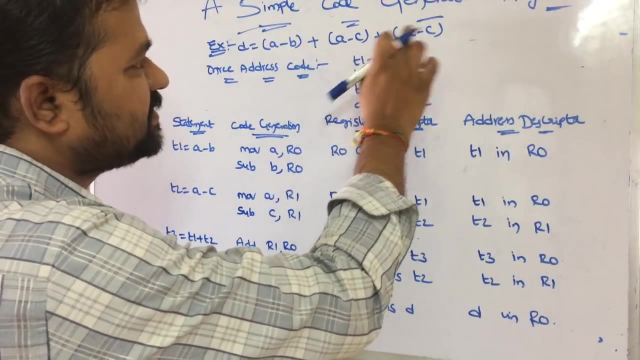 So this is a simple code generator algorithm. Now let us see an example for a simple code generator. Here the instruction is: d is equal to, within the parenthesis a minus b, plus within the parenthesis a minus c, plus within the parenthesis a minus c. 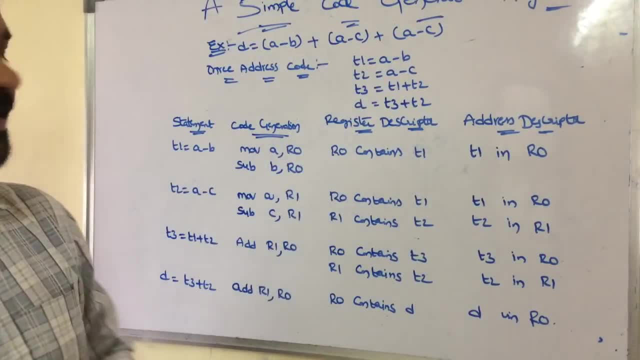 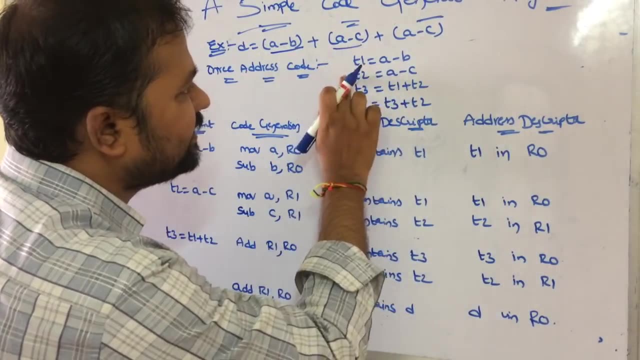 So first we have to write in three address code form. So t1 is equal to a minus b. Next one, t2 is equal to a minus c. Next, what is t3? t1 plus t2.. Next, d is equal to. 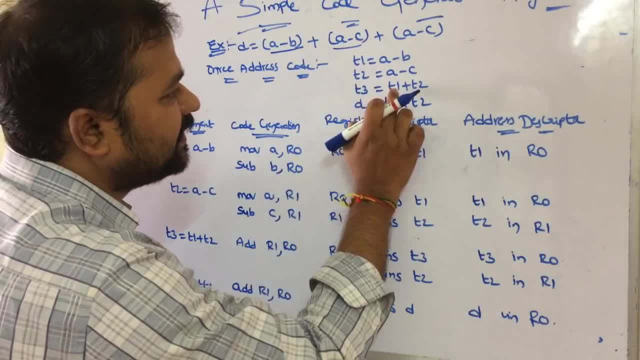 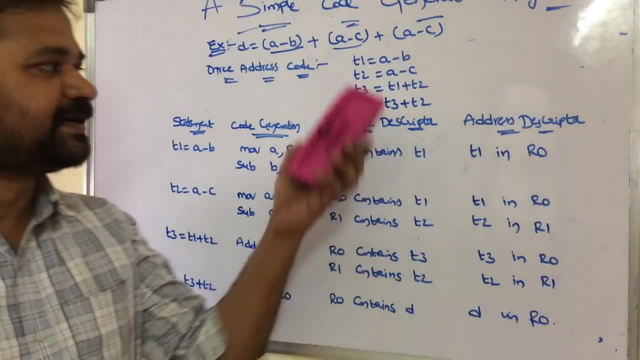 So a minus b plus a minus c is nothing but this t3. plus what is this? a minus c, a minus c is nothing but t2.. So this is nothing but three address code for this instruction. Now let us generate the code. 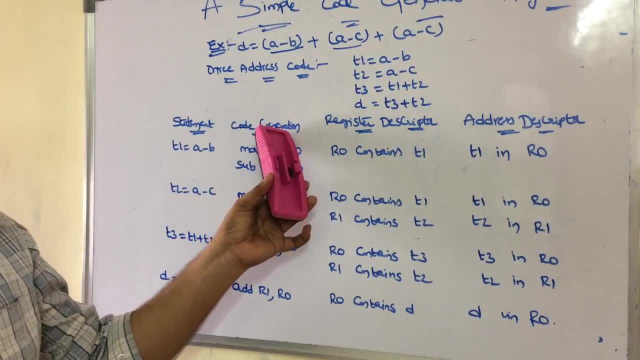 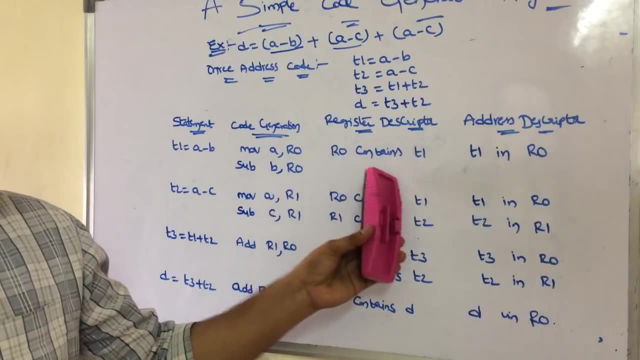 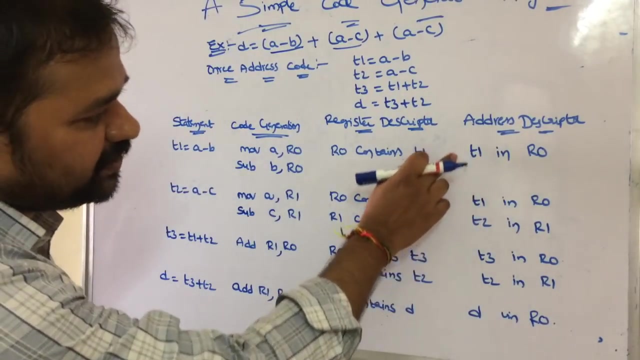 Here we have three columns: Statement code generation, register descriptor, address descriptor. So register descriptor specifies which register contains which variable, Whereas address descriptor contains the location where the variable is stored. So here the variable is stored in some registers. 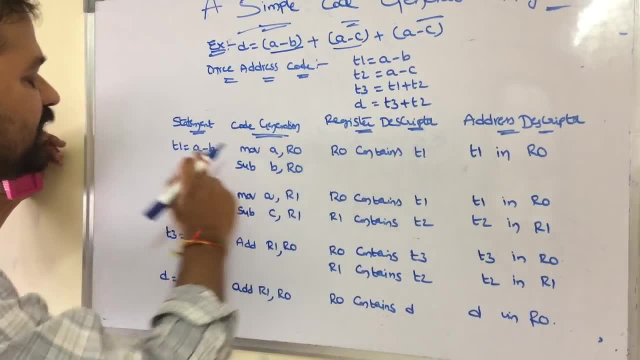 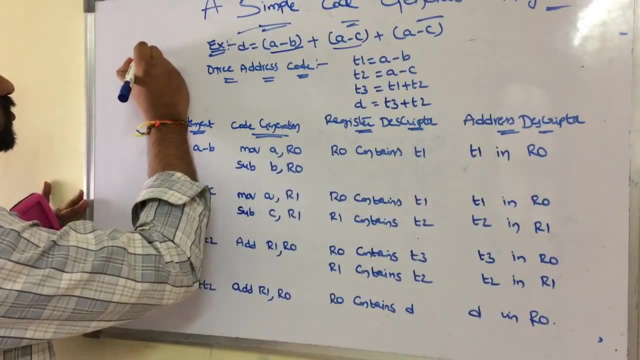 Now let us take the first instruction. t1 is equal to a minus b, So first we have to move a to some register. So move a. comma r naught. So now r naught contains a. Next one sub b, comma r naught. 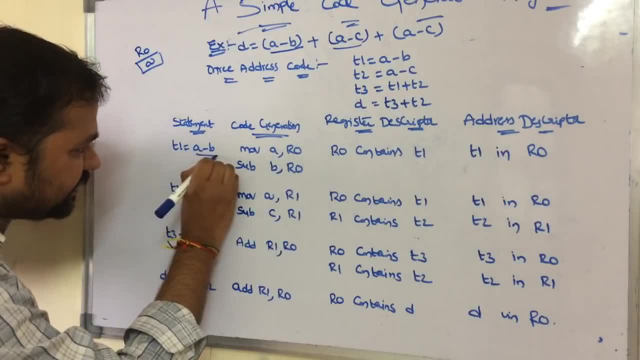 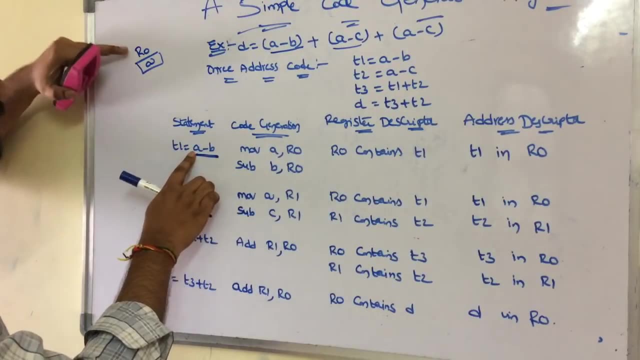 So what is r naught? Because here, what is the instruction here? t1 is equal to a minus b is the instruction here. So we have to subtract b from a, But a is available in r naught, So sub b comma r naught. 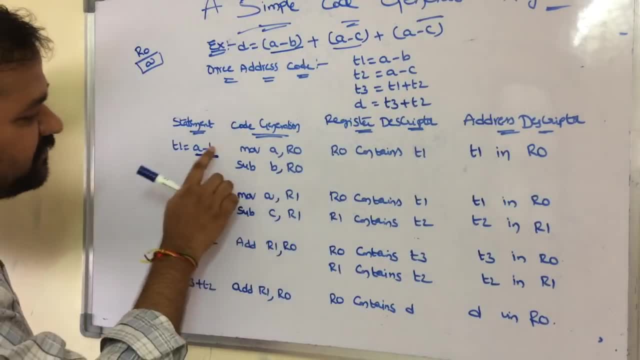 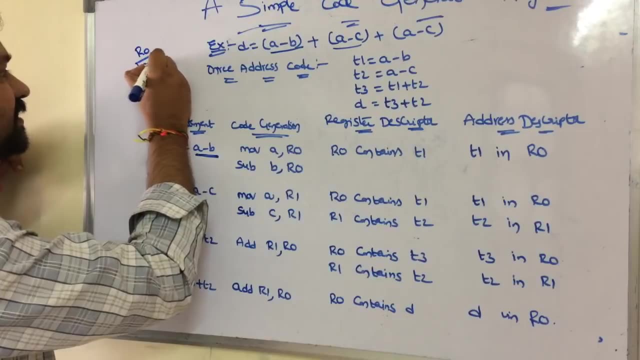 So now what will happen? r naught already contains a, So b will be subtracted from a. So now r naught contains the result of a minus b. r naught contains the result of a minus b, So we have to assign that result to t1. 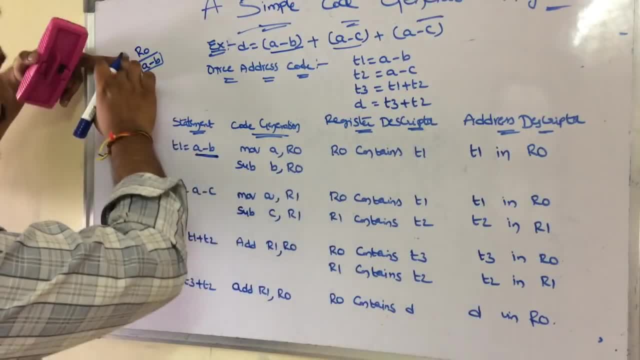 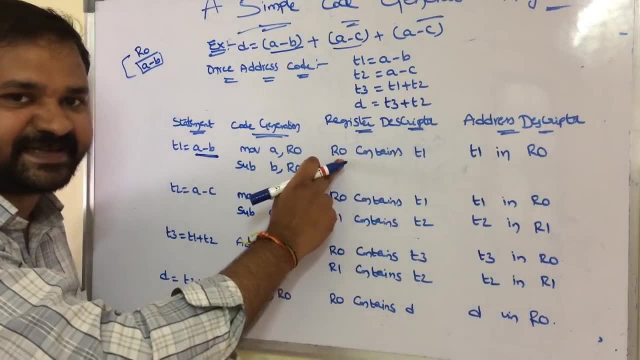 Okay, So what is register descriptor? now? r naught contains a minus b. So what is a minus b? t1.. So r naught contains t1.. That is register descriptor. Which register contains which variable? So r naught contains a minus b. 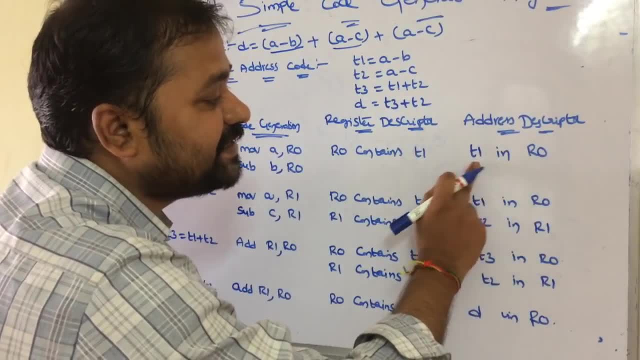 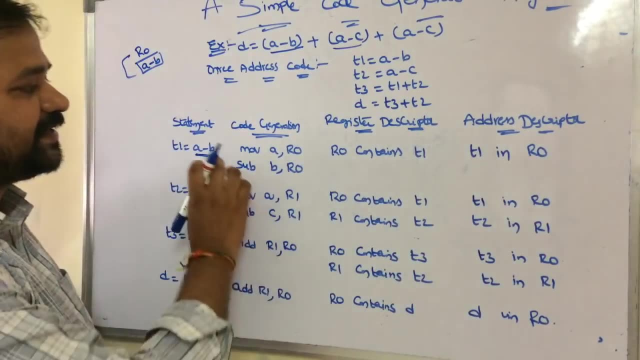 That is nothing but t1.. Whereas what is address descriptor? It contains the location where the t1 is stored. So here the t1 is stored in r naught, So t1 in r naught. So that is the first instruction code generation. 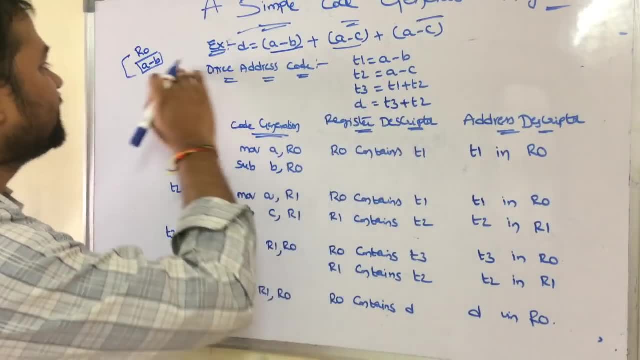 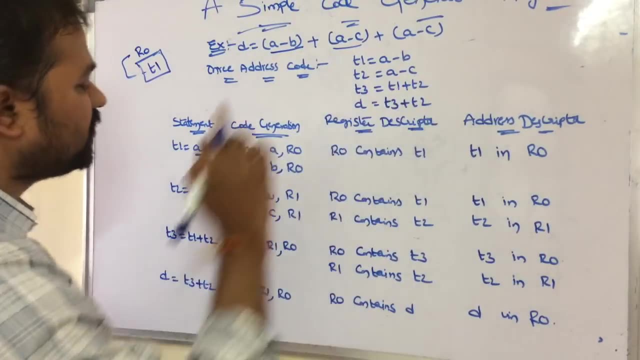 Now let us see the second instruction. What is the second instruction Here? the first instruction, r naught contains t1.. What is the second instruction? t2 is equal to a minus c, So t2 is equal to a minus c. 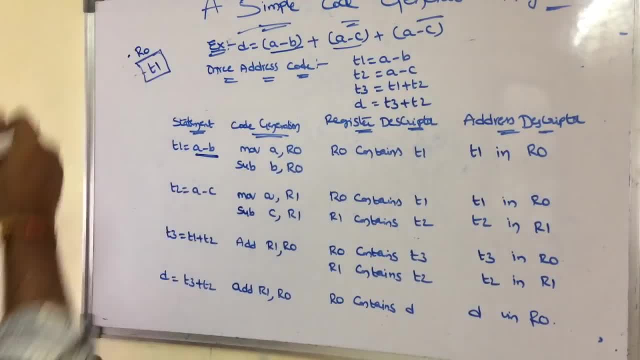 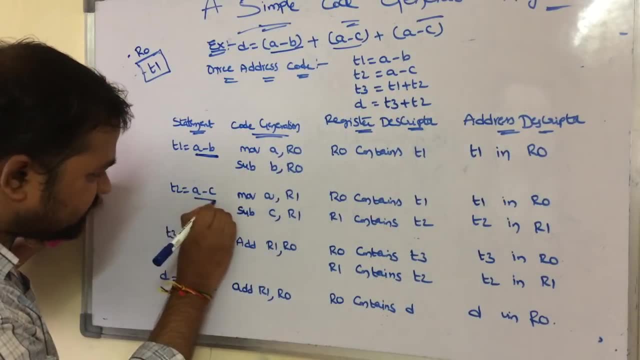 Here r naught is not free. It already contains t1.. So we need to take one more register. So let the next register is r1.. So move a comma: r1.. Because here the instruction is a minus c. 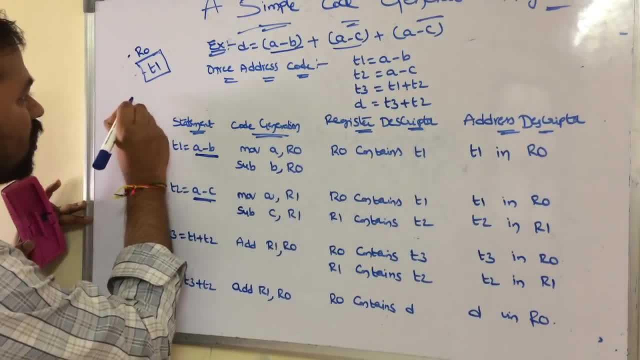 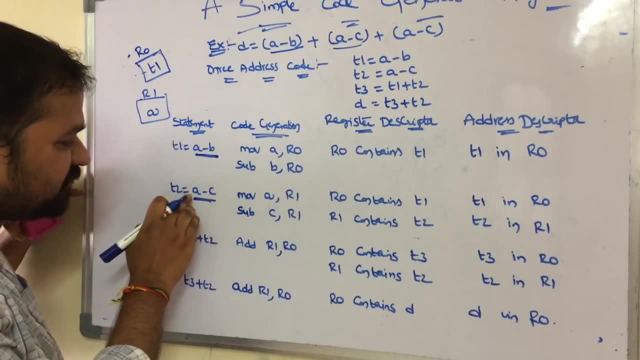 So a is moved to r1. now a is moved to r1.. So now r1 contains a Next one. we have to subtract c from a. We have to subtract c from a, But already a contains r1.. 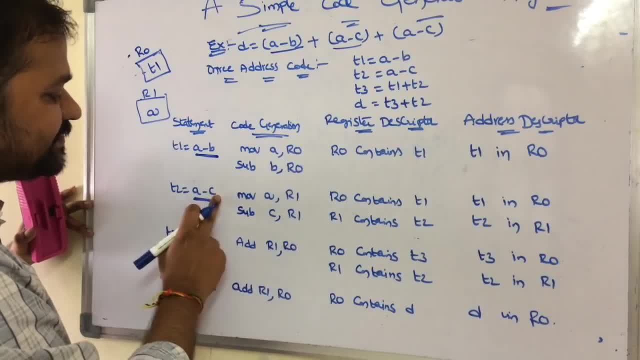 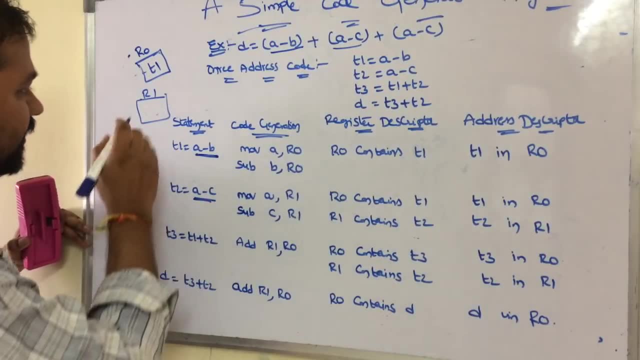 So sub c comma r1.. So now what will happen? c will be subtracted from a and the result is stored in t2.. So now, what is r1?? r1 contains a minus c. a minus c is nothing, but the result is assigned to t2.. 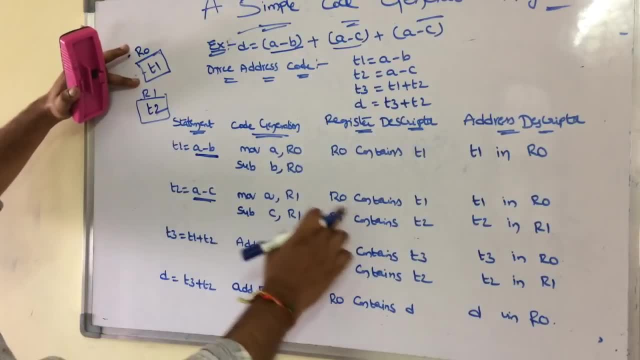 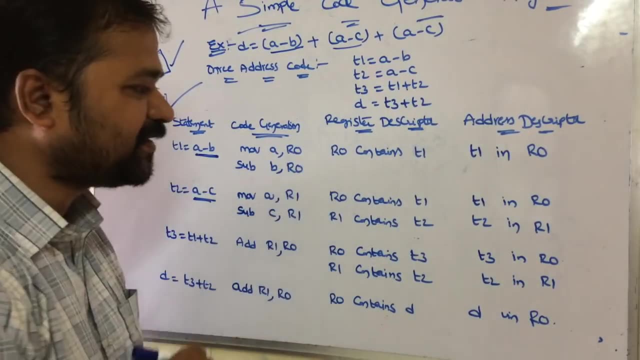 Now let us see the address descriptor. So r naught contains t1.. This is the first statement. Second statement: r1 contains t2.. So this is the second statement. So this is about register descriptor. Now let us see address descriptor. 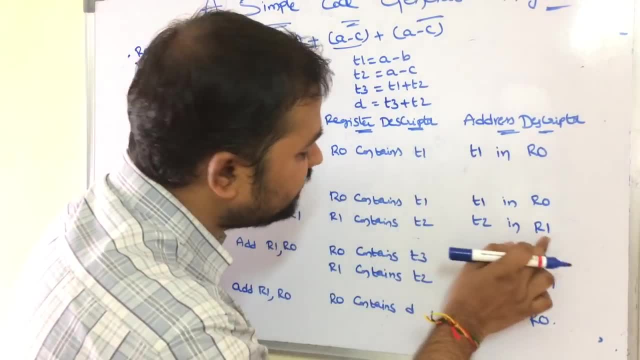 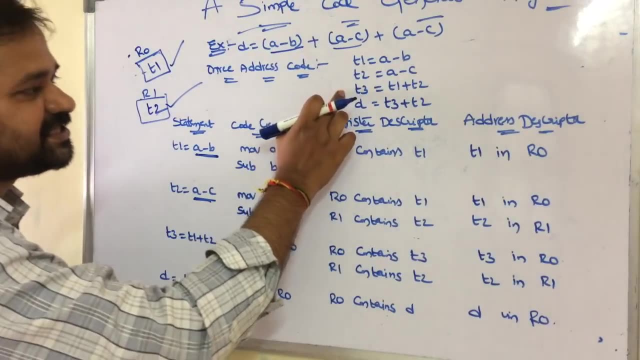 So t1 is stored in which location r naught t2 is stored in which location r1.. So this is nothing but address descriptor information. So this is the second instruction code. Now let us see the next instruction. 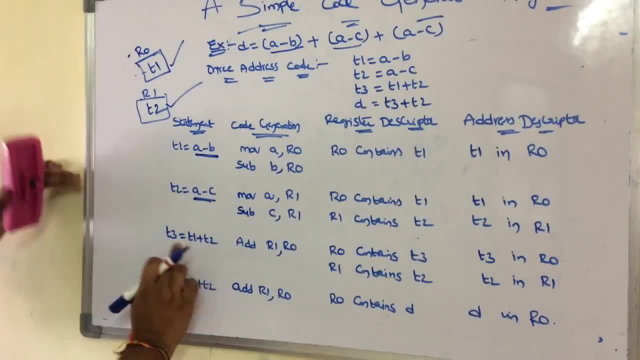 t3 is equal to t1 plus t2.. t3 is equal to t1 plus t2.. So t1 resides in r naught, t2 resides in r1.. So we add r1 comma, r naught. It is our choice. 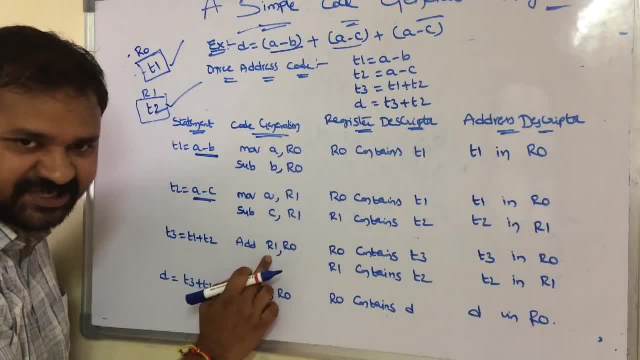 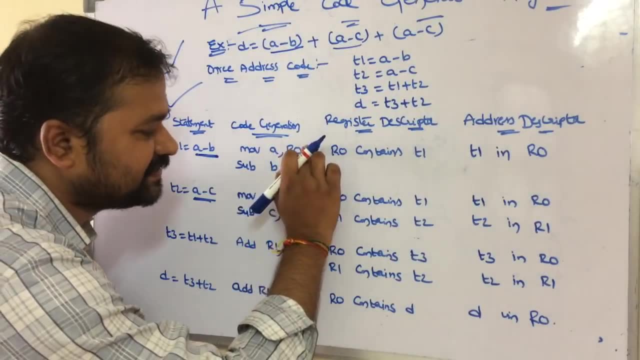 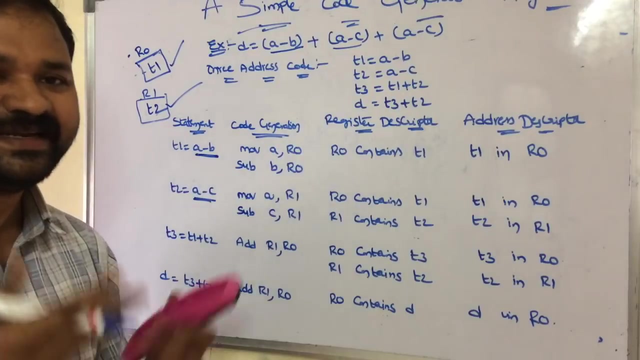 We can write here: r naught, comma r1, or we can take the first one as source register or the second one as source register. It is our choice Here. in this example we have taken the second one as destination register. If we want, we can take the first one as destination, also by writing: move r naught, comma a. 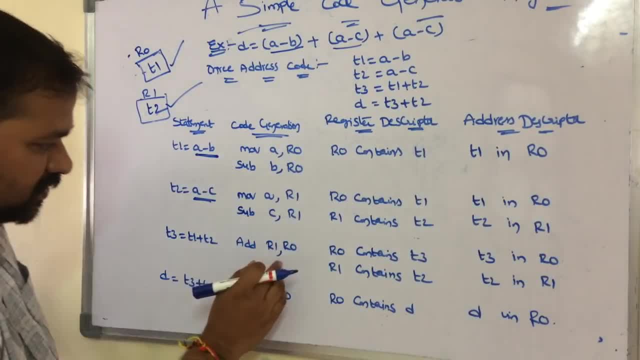 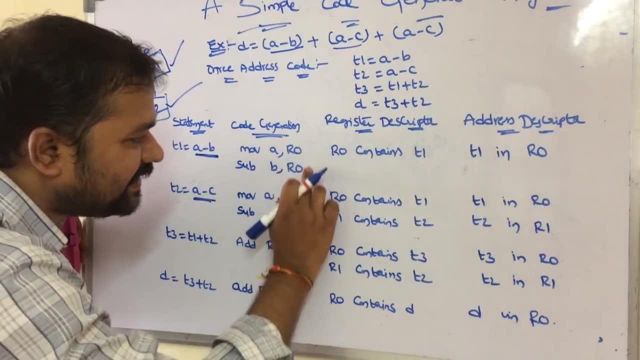 It is our choice. We can write in any manner as we like. So now we add r1 comma, r naught. So r1 and r naught will be added, And here we have taken the second one as destination register. 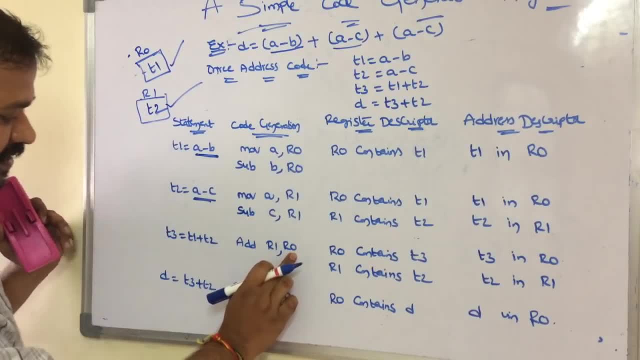 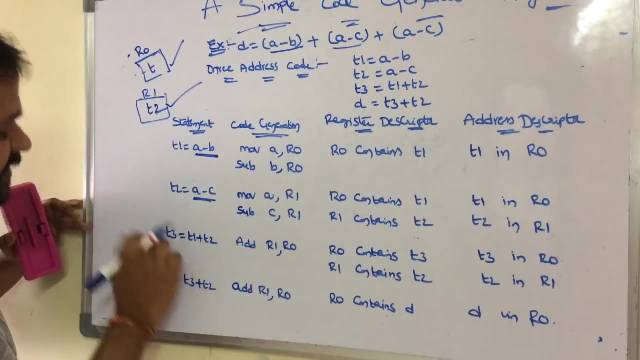 So r naught contains the result of r1 plus r naught. So r1 plus r naught is nothing but t1 plus t2.. So now r naught contains the result of t3.. Now let us see here register descriptor. 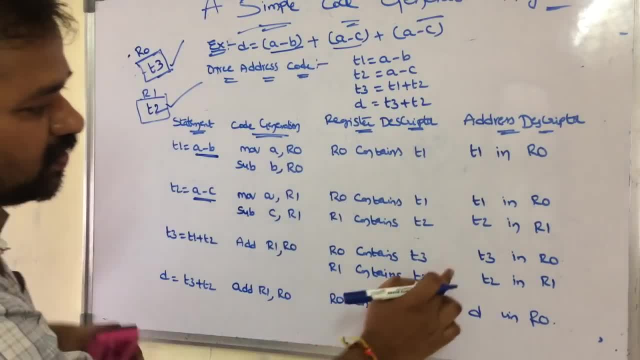 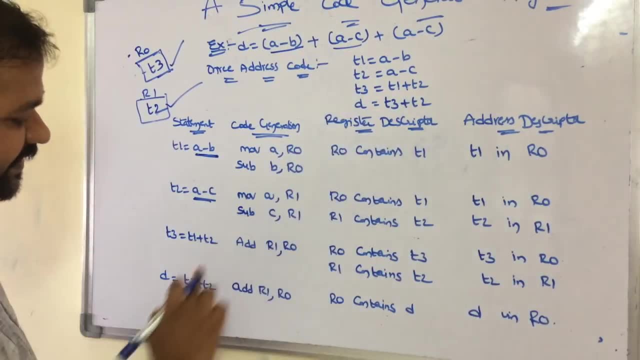 r naught contains t3.. r1 contains t2.. Now t3 is available in r naught. t2 is available in r1.. Now let us see the last instruction code. So d is equal to t3 plus t2.. 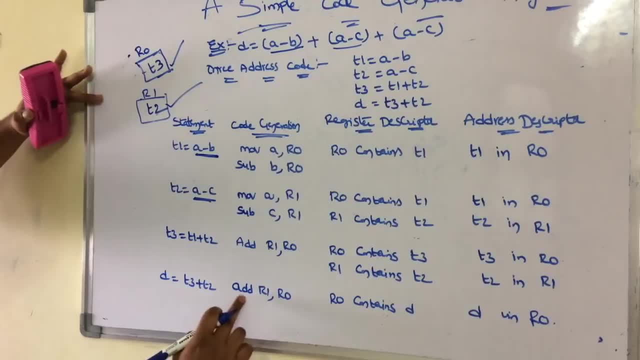 So t3 is available in r naught. t2 is available in r1.. So we add r1 comma r naught. Now what is the next instruction Here? the result is available in r naught, So we have to move that result to d. 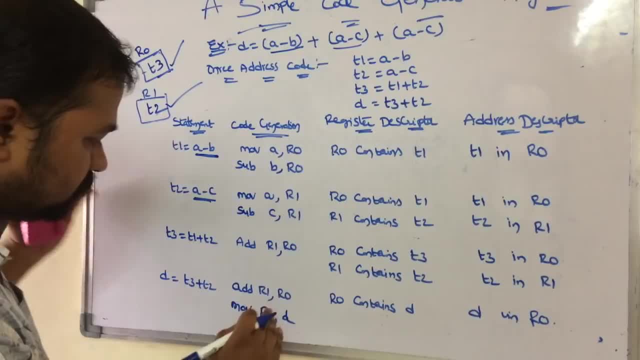 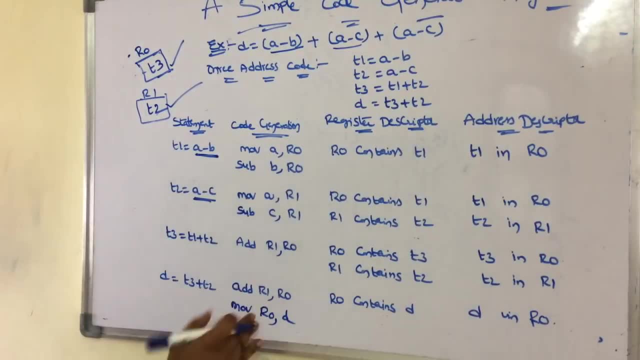 So move r naught, comma d, So we add r1 comma r naught, So r naught contains this result now. So r naught contains d, So already r naught contains d, So there is no need of moving here. 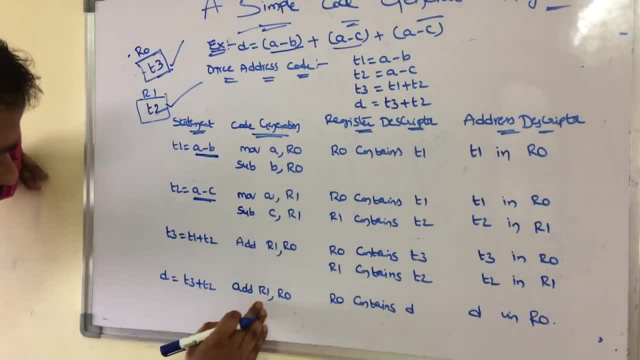 So we add r1, comma, r naught. So what will happen now? So what is r1? t3.. What is r1? t2.. r naught t3.. So t3 and t2 are added and the result is stored in d.